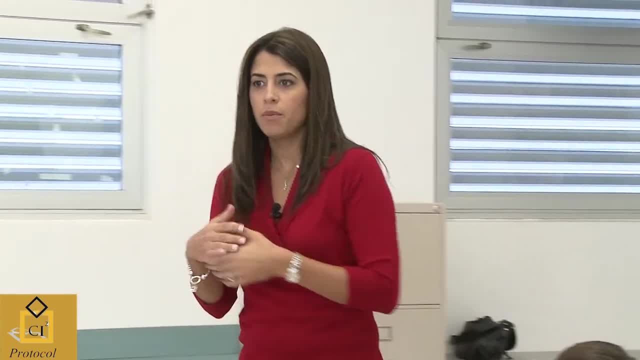 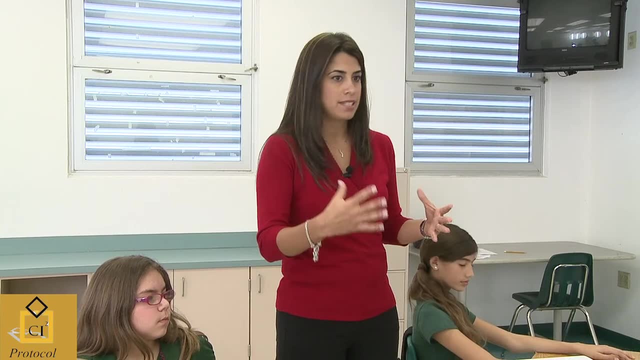 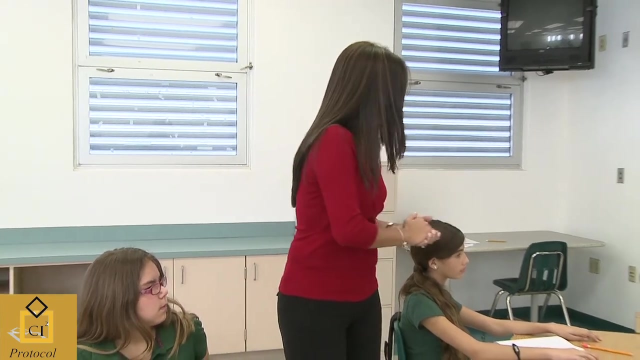 unit rate. No, Most of the time when you buy things, you buy them with several, You don't just buy one, You buy a package usually that has several items. Let's talk about how. about a sports drink package that you have? what like, how many? Or mixed goodies, Or mixed. 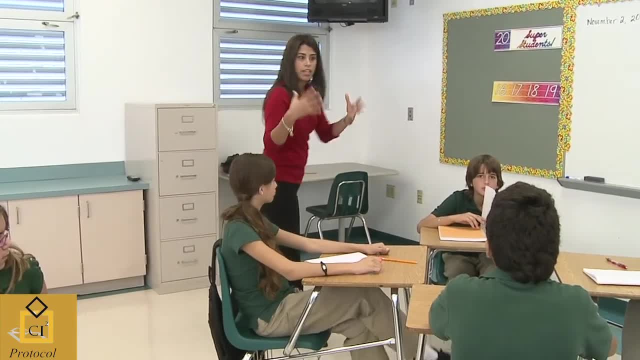 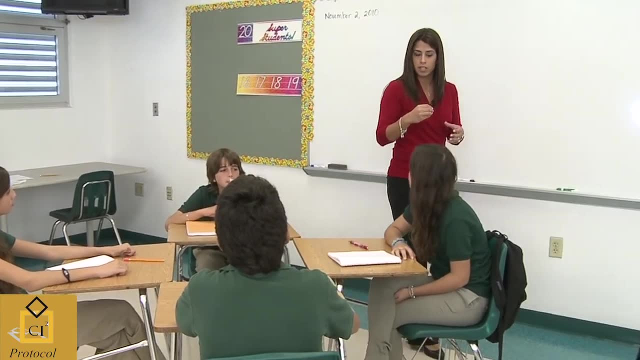 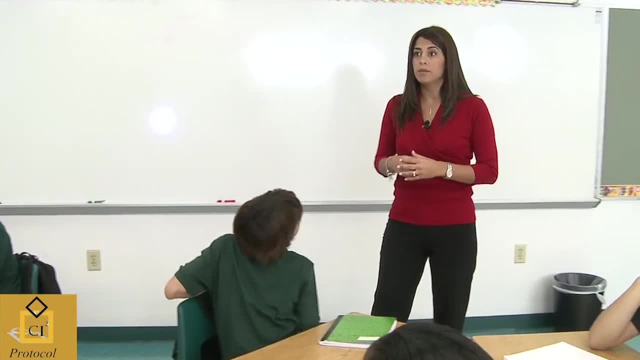 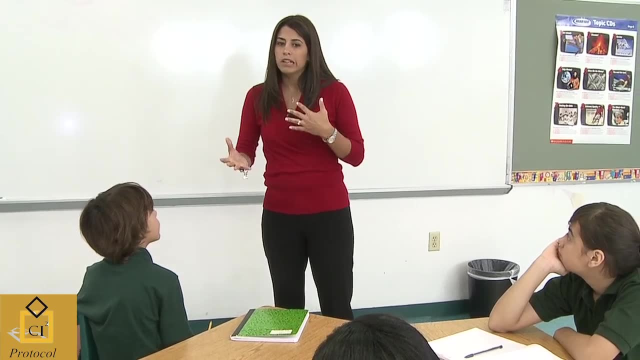 Or canned sodas. Okay, Well, some, like I was saying before, some of the supermarkets have a little label that say what the unit rate is. Okay, So pretty much we're going to learn a little bit about how you can tell if your parents are getting a better deal If they shop, maybe at a wholesale. 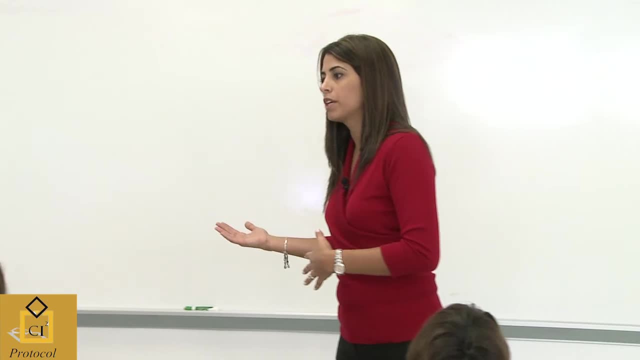 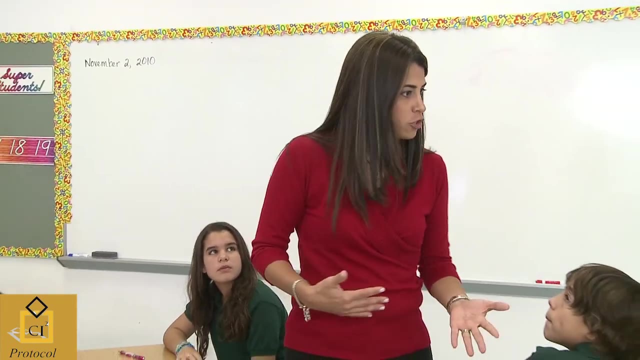 club, Or if they're getting a better deal at a wholesale club, Or if they're getting a better deal at a local supermarket, But not only that. have you ever wondered, maybe, if you're on a track team at school and who's the faster runner Depending on how many laps you run? Okay, I bet. 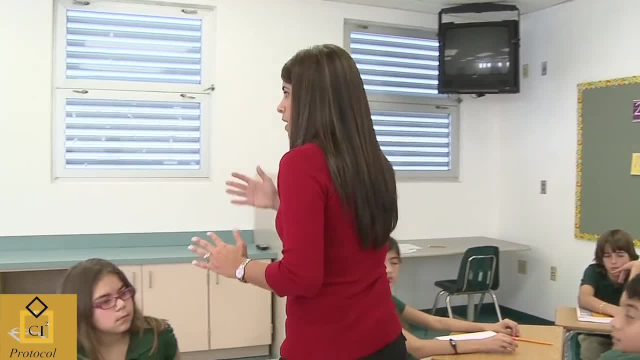 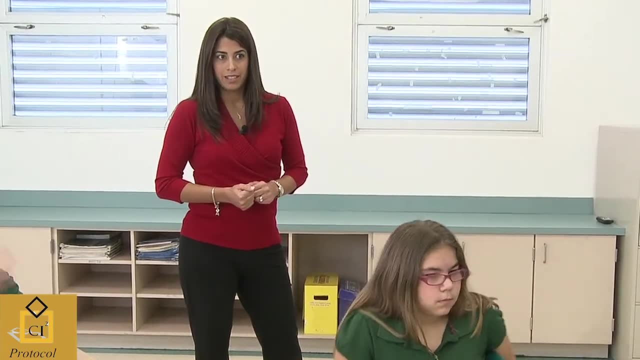 you guys are really good And you can tell automatically. just by watching the race You can tell who the faster runner is right. How many of you are fast? Yeah, Okay, Now I'm going to ask this question: How many of you are fast, short distance? 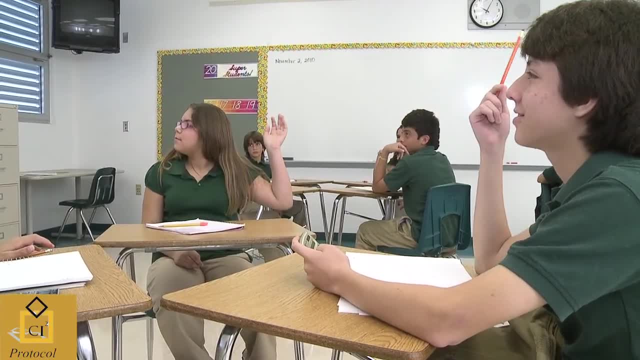 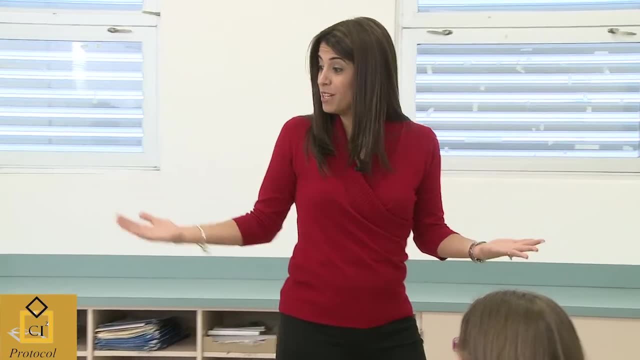 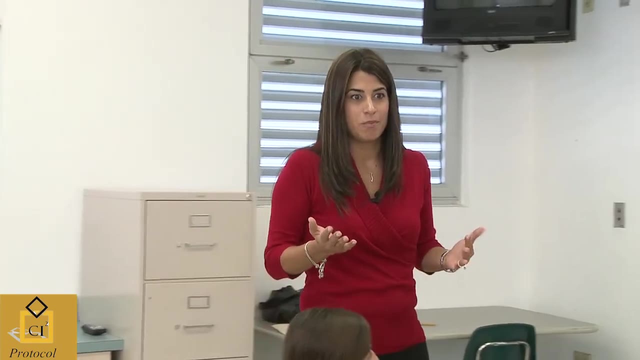 How many of you are fast? long distance, Okay, Did you see the difference there? So maybe over time, over a certain amount of distance, you know, maybe Britt and Sergio you might win the race, But if it's a short distance, maybe Lazaro will win the race. Okay, So we're going to start. 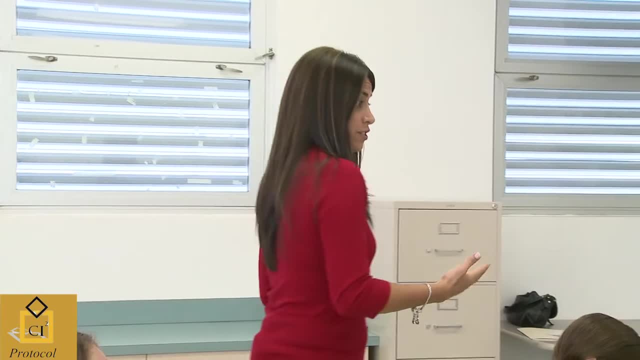 learning about this and learning about unit rate and ratios- My main objective when I was teaching the lesson. how many of you are fast long distance? How many of you are fast short distance? Okay, So we're going to start learning about unit rate and ratios. Okay, So we're going to start. 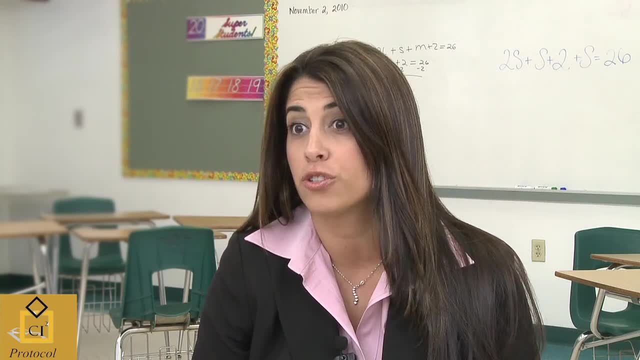 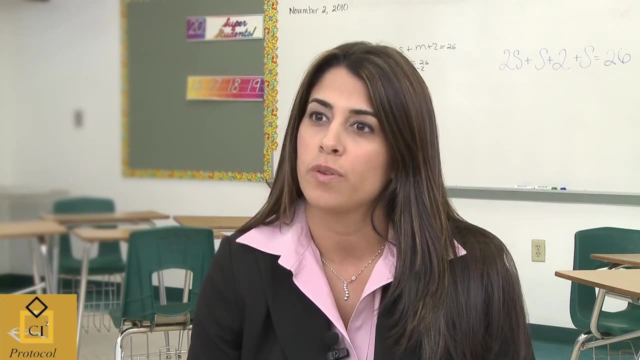 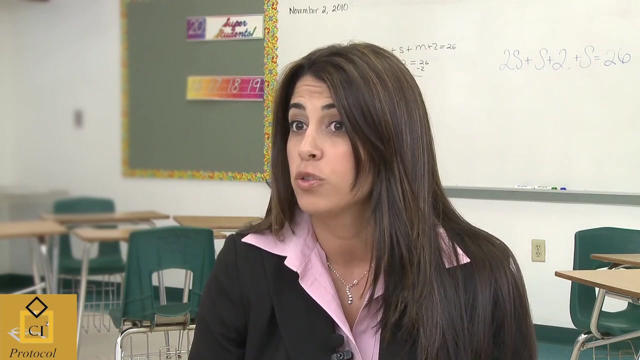 comparing ratios. I really wanted the students to understand how to compare ratios. I wanted them to be able to know how to use the correct mathematical vocabulary, not simply by giving them a definition for ratio, but linking it to real world, And that's why I incorporated the kids 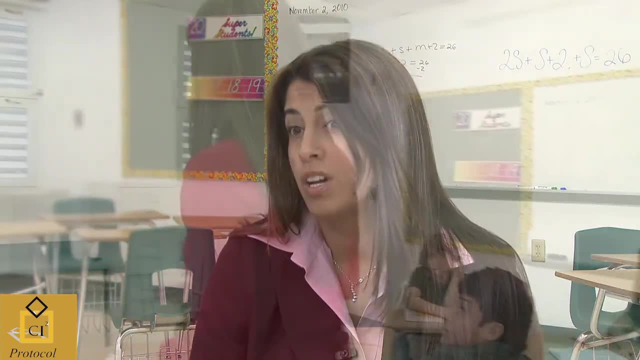 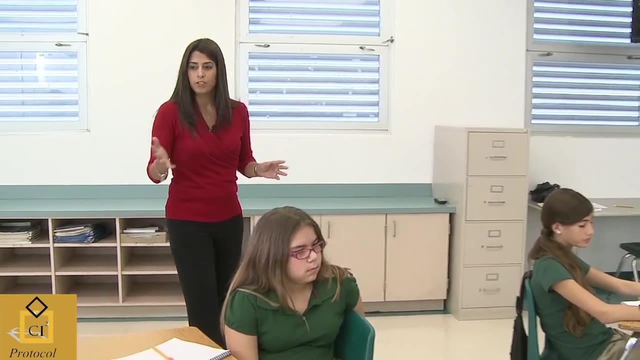 when I was trying to teach them a ratio. And you can tell automatically. just by watching the race. you can tell who the faster runner is right. How many of you are fast? Yeah, Okay, Now I'm going to ask this question: How many of you are fast? 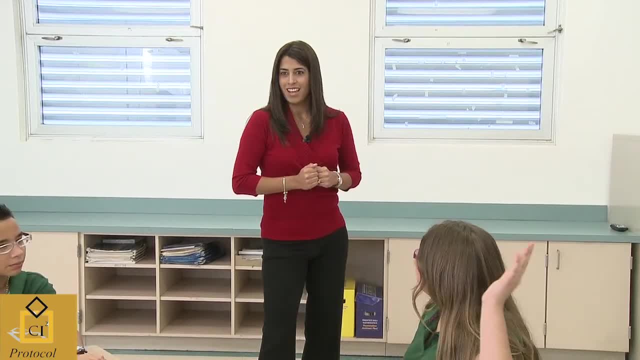 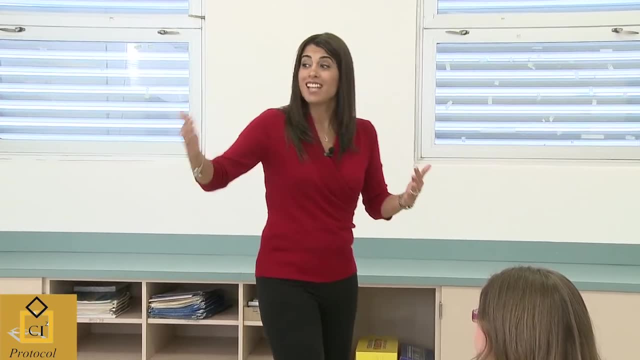 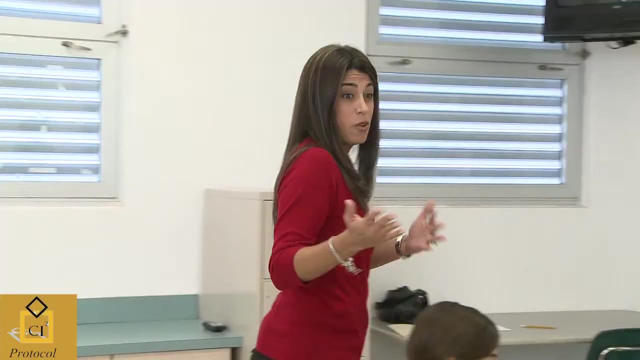 short distance. How many of you are fast? long distance, Okay, Did you see the difference there? So maybe over time, over a certain amount of distance, you know, maybe Britt and Sergio, you might win the race, But if it's a short distance, maybe Lazaro will win the race. 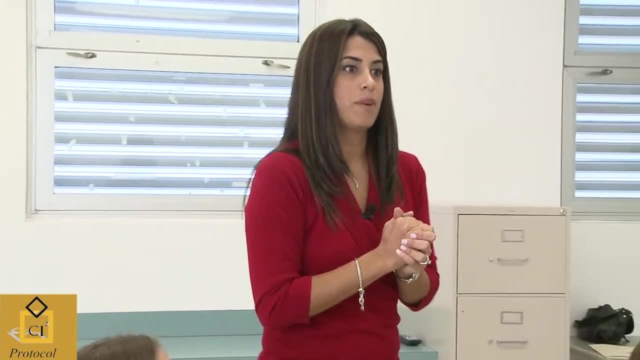 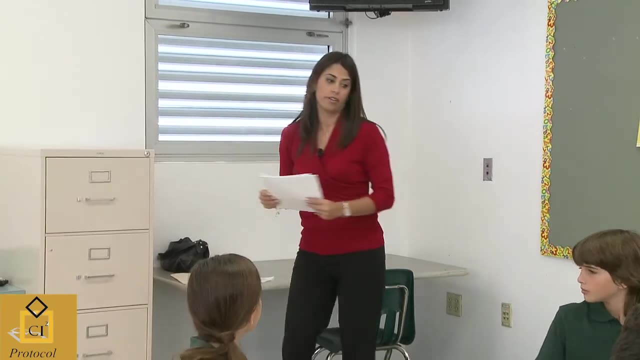 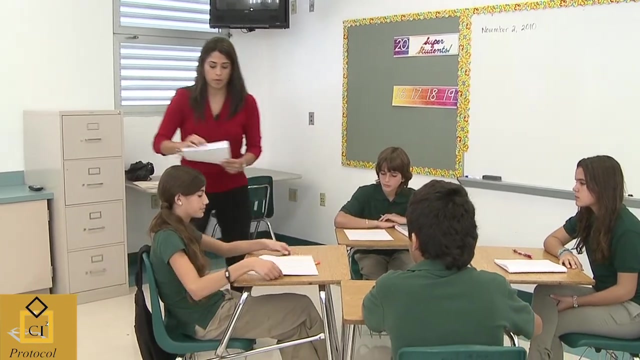 Okay, So we're going to start learning about this and learning about unit rate and ratios. I'm going to start off by giving you a worksheet. I want you to analyze one of the problems together And I'm going to give you some time to analyze it. Give one to each one of your group members, please. 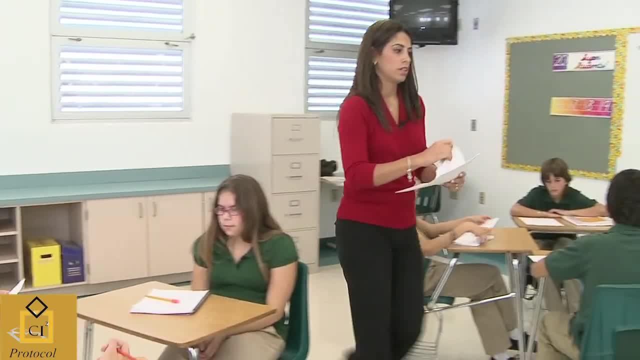 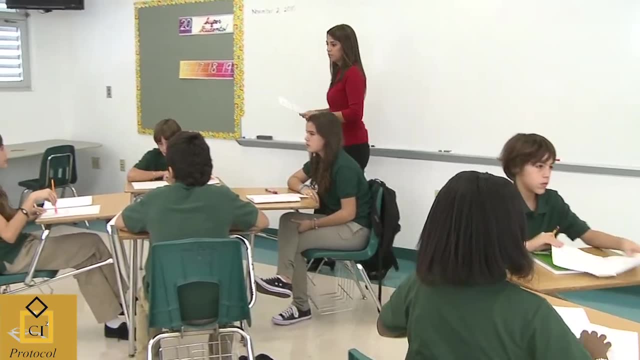 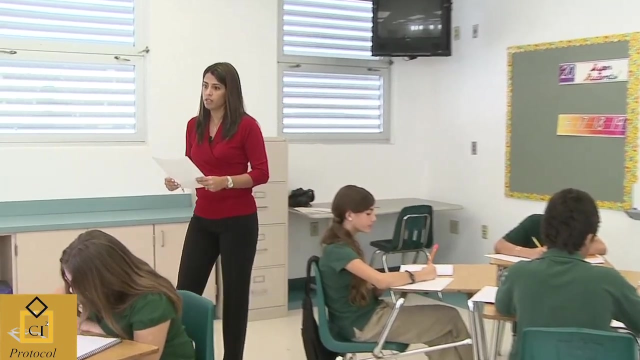 Lazaro, give one to each one of your group members. Britt, give one to each one of your group members, please. Amanda, Yes, please put your name at the top of the paper And let's take a look at number one. 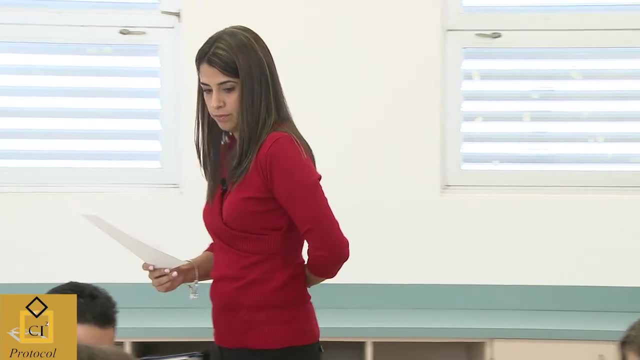 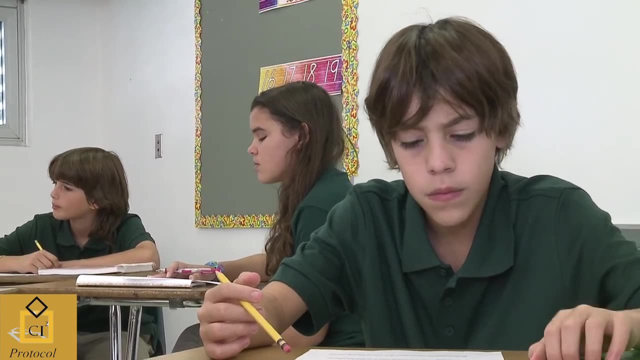 David, can you read that for me please? Ariel can run four laps in 12 minutes. Susan can run three laps in nine minutes. Who is the fastest runner? Okay, Let's really understand what the problem is asking. What is the problem actually? 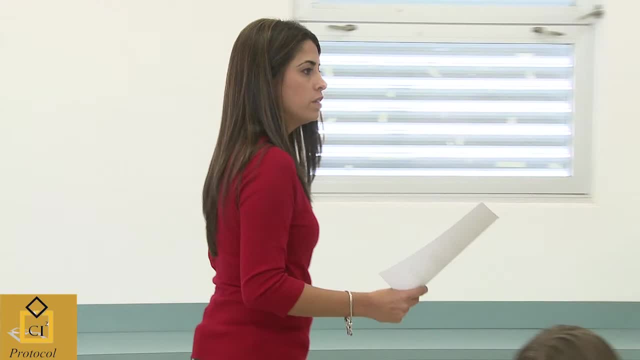 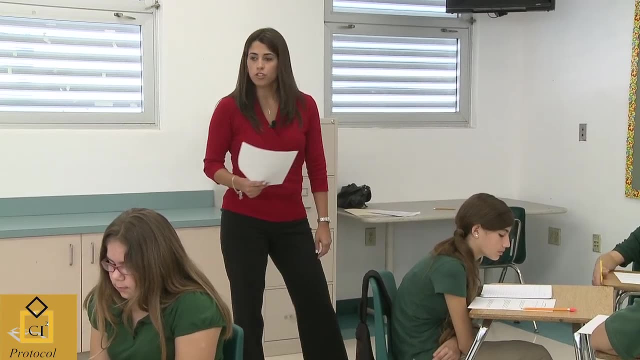 What is the problem actually asking Allie Who is the fastest runner? Who is the fastest runner Between Ariel and Susan? Very good, Very good. Now what I want you to do is I want you to discuss this problem with your group members. okay, 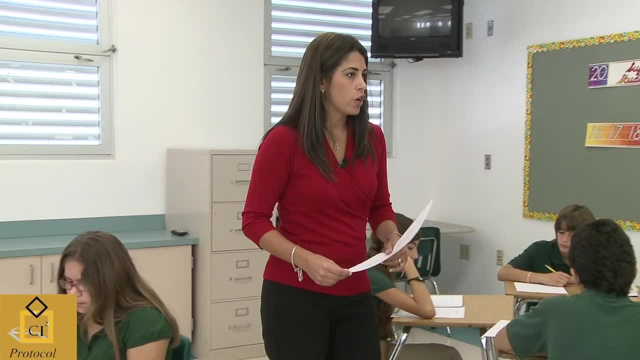 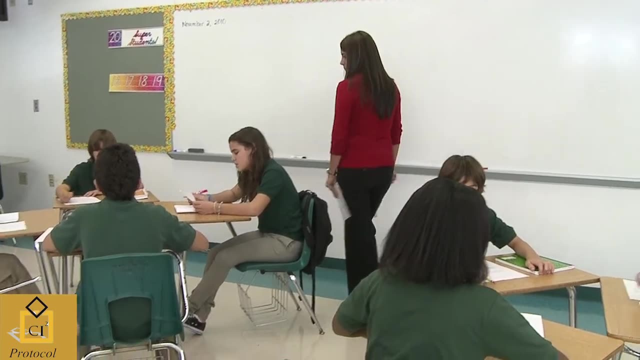 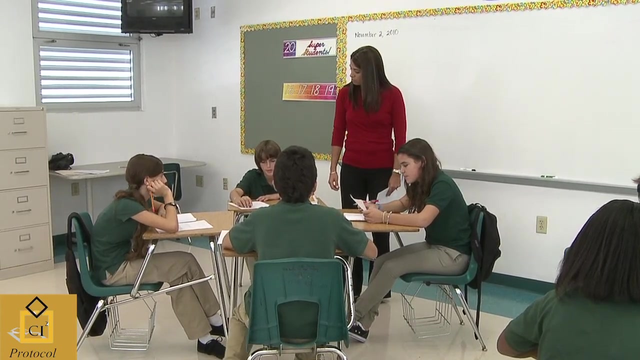 Take a minute to figure out how to solve it and then share with your group members how you solved it. Let's take a few minutes- three or four minutes- to solve that problem together. How do you figure out? they're both the same. 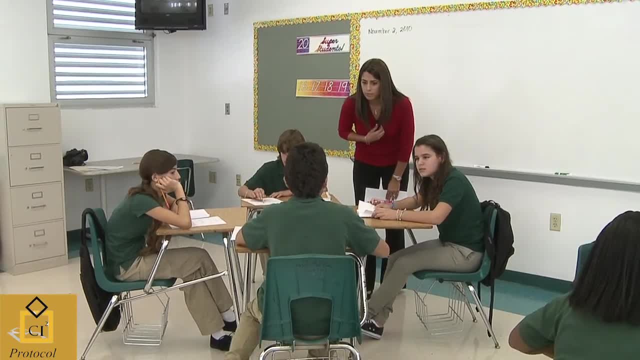 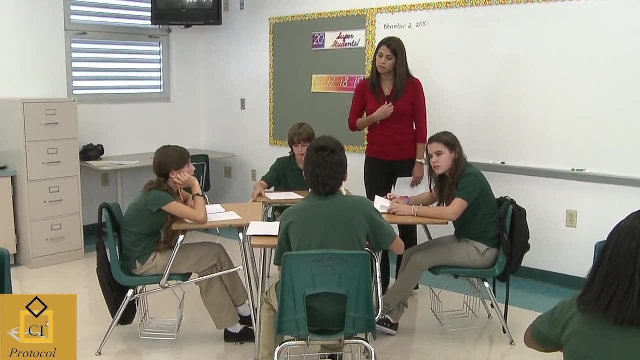 How do you figure out they're both the same? The way I would figure it out is I take the actual two numbers and I divide them, So then one lap every time. I deal with it for three minutes, So then I figure out how much time is one lap. 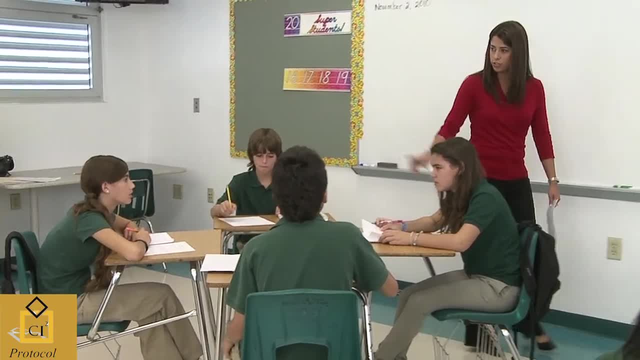 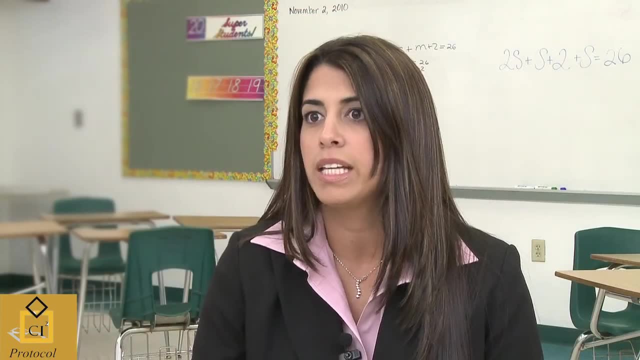 Look and see, because I think Allie and Amanda are still not understanding. Explain it to them, Show it on paper. maybe I really do believe in cooperative groups. It gives me the opportunity to walk around to informally assess the students. 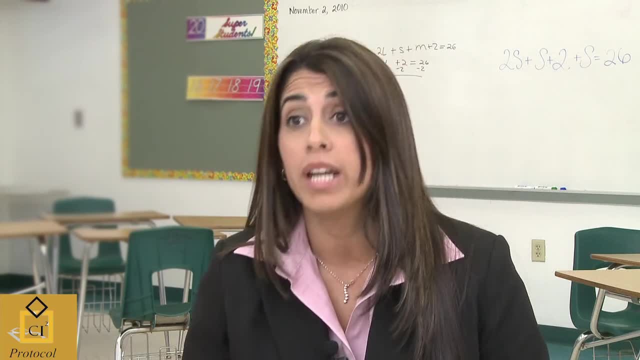 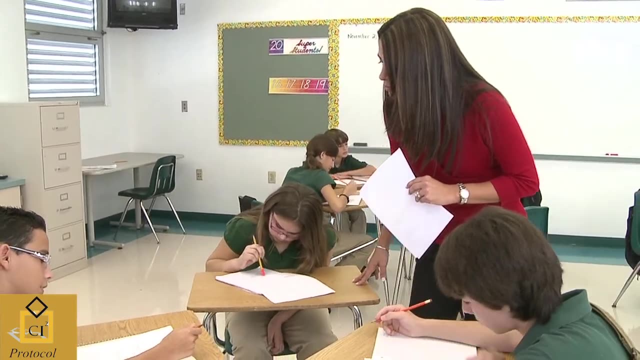 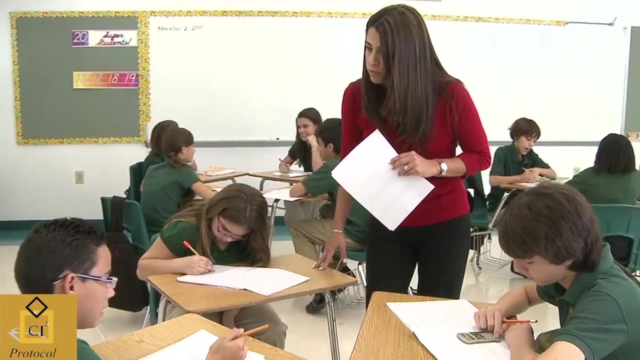 and that way I can see where to go next, or perhaps maybe differentiate the instruction at that time, based on the information that I'm gathering as I walk around. It's very important to provide different varieties and opportunities for students to interact with each other. I have seen some very unique ideas come out. 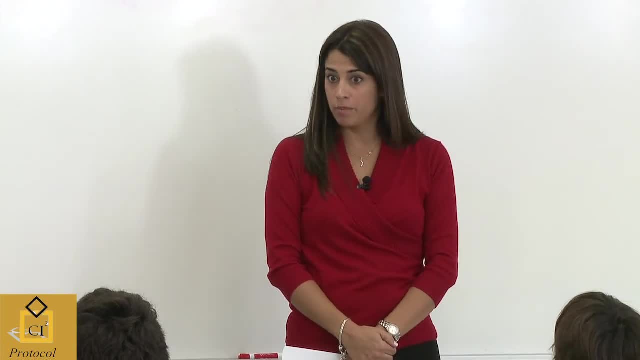 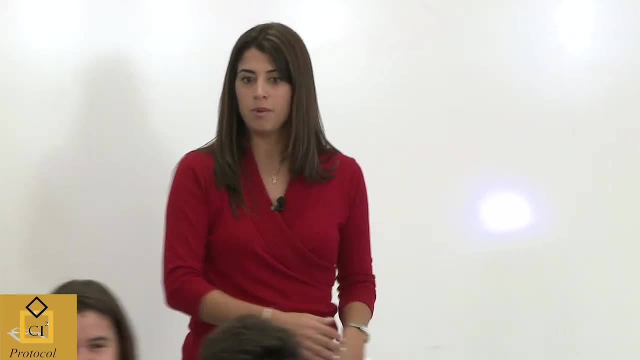 and I'm going to ask for your input. I'm going to ask your group to pick a member to explain which way you chose to answer this question. Let's see if you came up with the right answer. Who would like to go first? 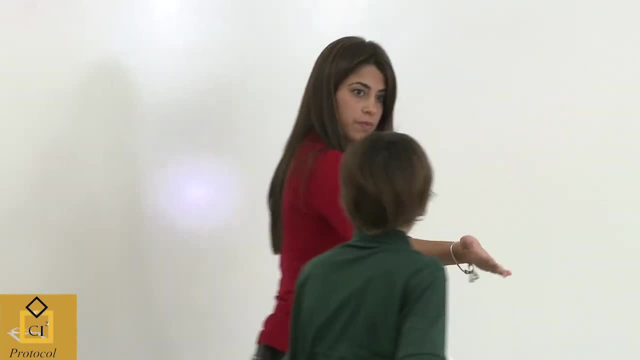 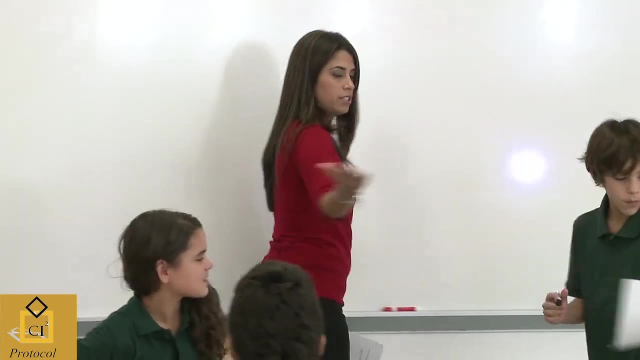 Next group discuss. You want to be the speaker for your group. Sure, You guys. okay with that Great, Go Show me explain to the class what your group decided to do. Well, the way I would figure it out is I would take the two numbers. 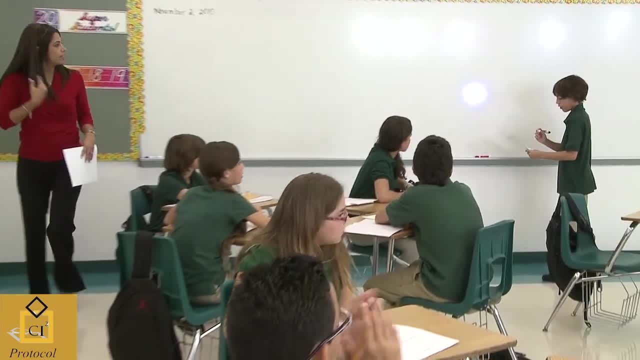 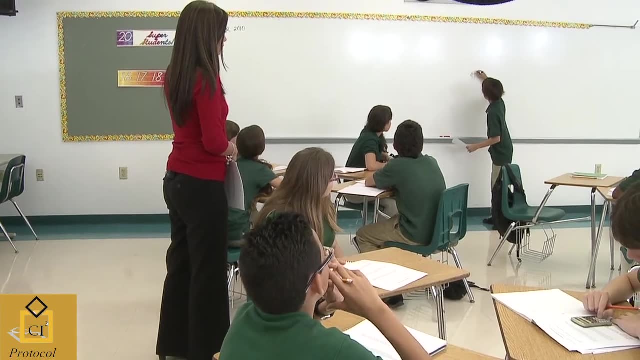 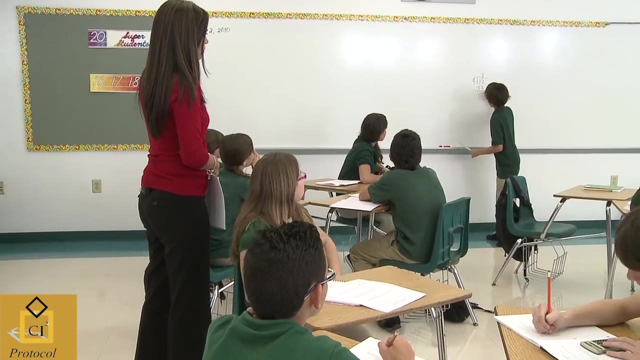 A little louder. Nick, What I would do, I would take the two numbers for Ariel, which is 4 and 12, and then I would divide them, which would be 3.. So that's how long Ariel would take to run. 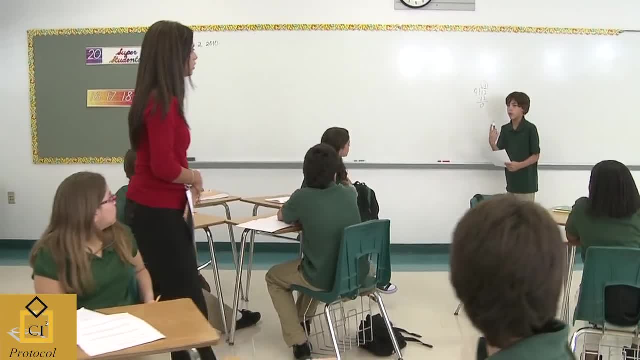 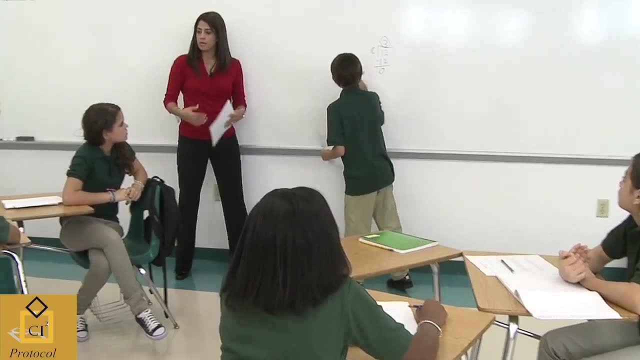 That's how many minutes it would take for Ariel to run one lap. Excellent. Can you identify? Can you write that sentence? or can you identify? Can you write one lap in three minutes? Ashley, that's what you guys came up with. 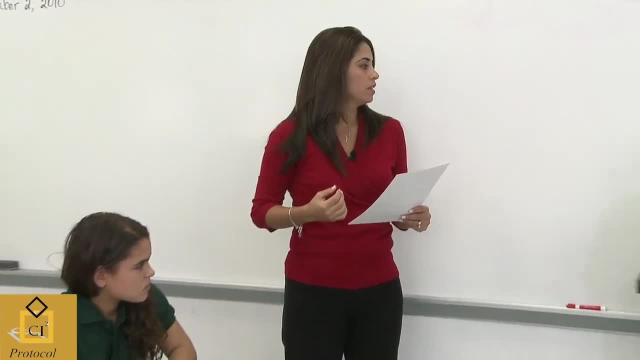 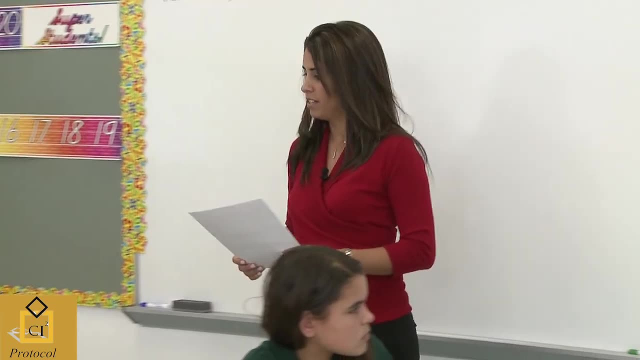 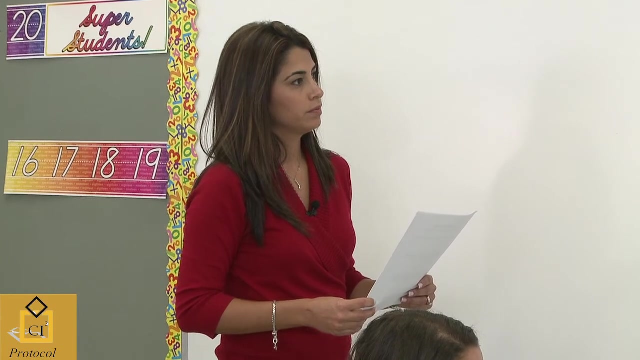 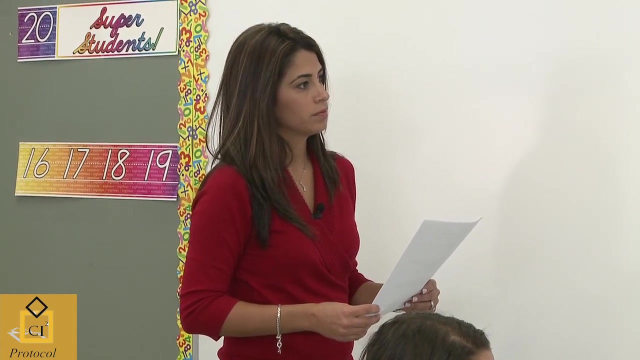 Excellent. Okay, And that's for: Oh, I like that you did that. That's for Ariel, Ariel, nice Identify Would be 3 divided by 9, which would be 3.. So again, it would be 3 minutes 1 lap. 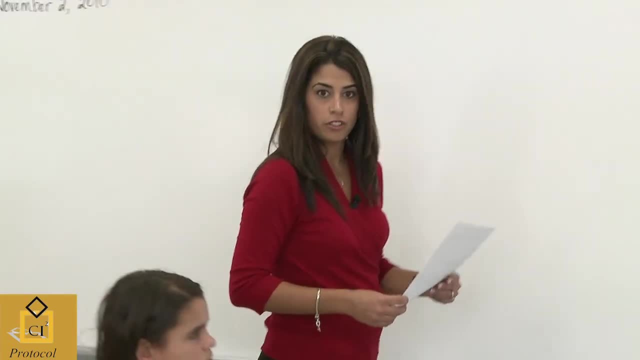 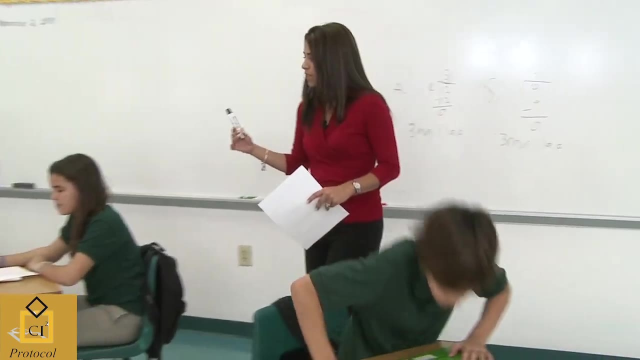 Nice job, Nice job, Excellent. You did a great job in this group. Okay, we're going to call another group up. Thank you for participating, Nick. We're going to call up Sergio's group And let me ask you: is your method the same way? 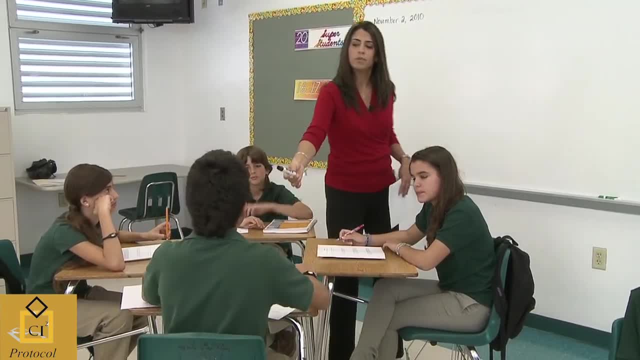 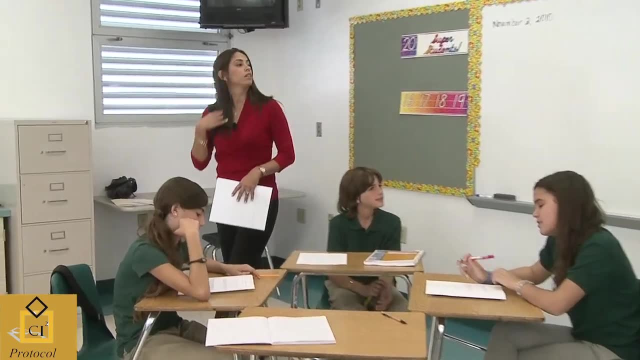 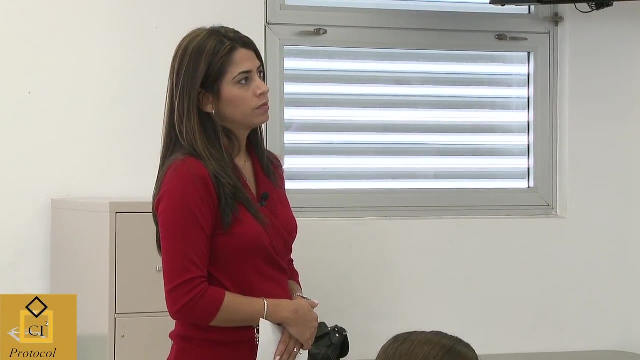 Did you solve it that way? No, I'm really curious. Let's see what method you chose. You all discussed it, right, You came up with a method. They're the same because like one lap in 3 minutes. 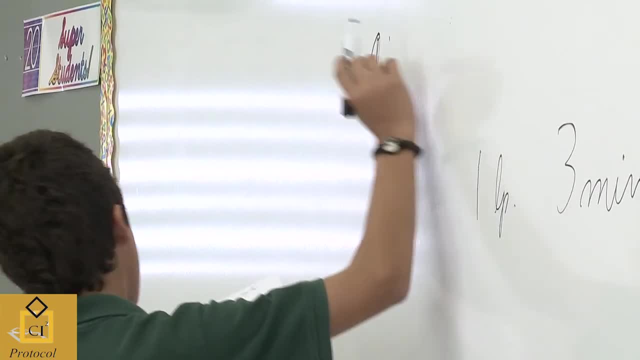 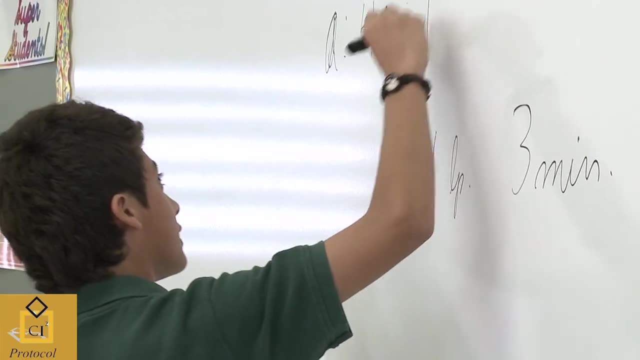 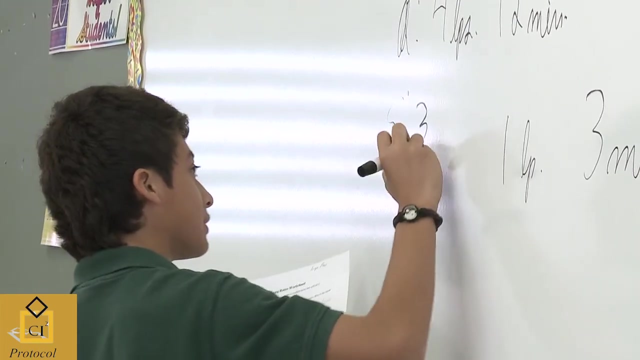 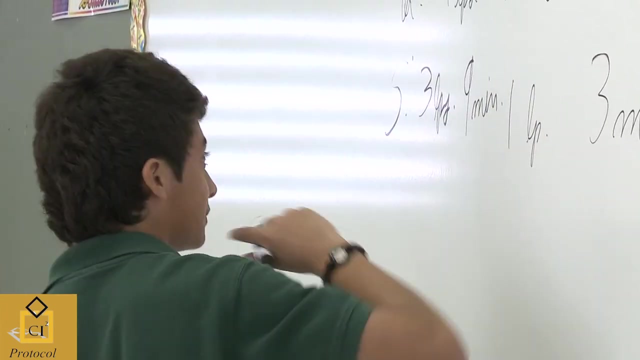 So Ariel ran 4 laps- same amount- in 12 minutes And Susan ran 3 laps in 9 minutes. Okay, so you have identified the information from the problem, Excellent, Yeah, So 1 lap is 3 minutes. 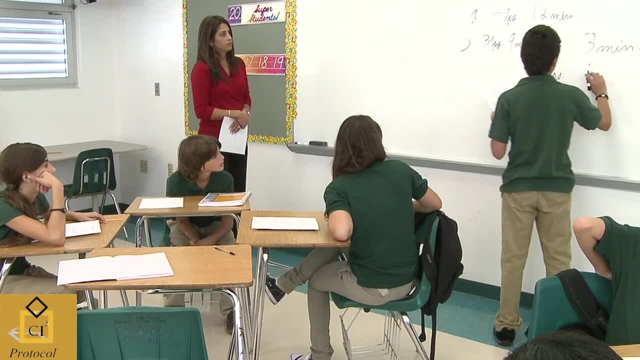 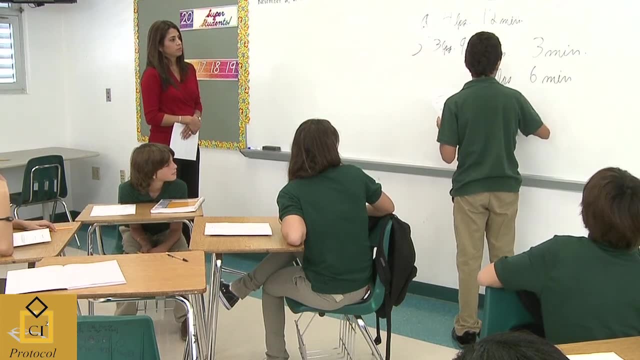 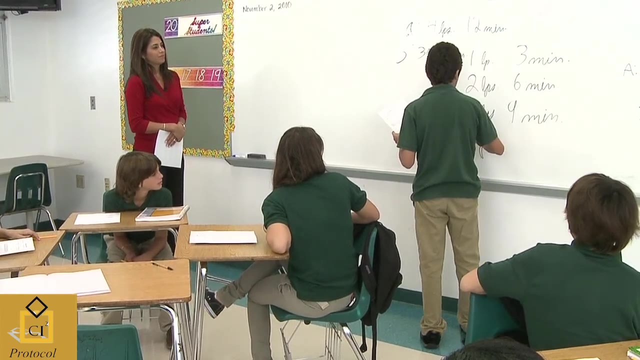 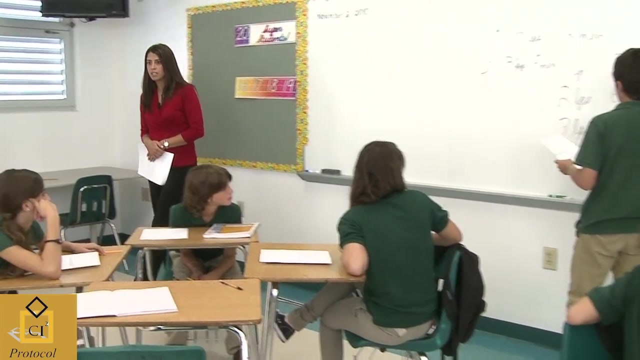 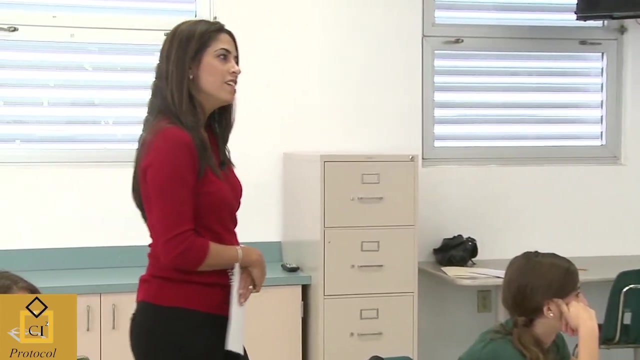 2 laps will be 6 minutes, 3 laps will be 7 minutes, Okay, And 1 lap will be 9 minutes And 4 laps will be 12 minutes. Wow, very interesting. So if Susan ran one more lap, she would have the same amount as Ariel. 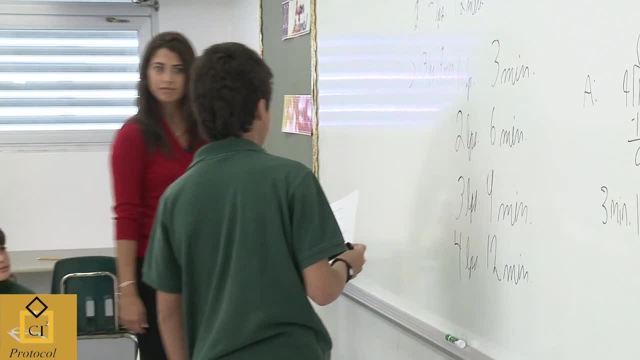 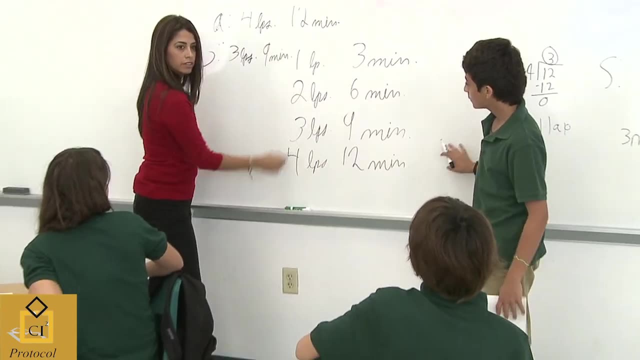 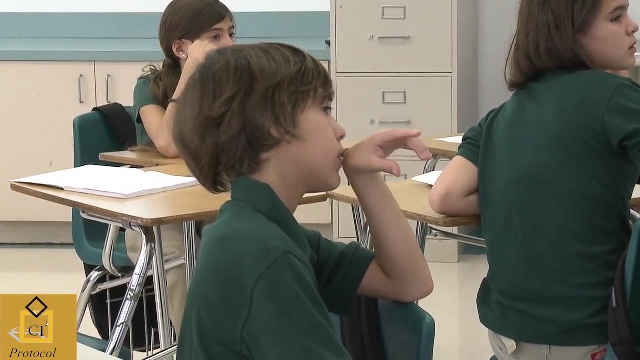 Very interesting. You've identified a pattern. When students explain how they solve the problem, they should be able to relay the steps they used and explain the mathematics behind their solution. As students progress through school, the mathematics behind their solutions should become more advanced.